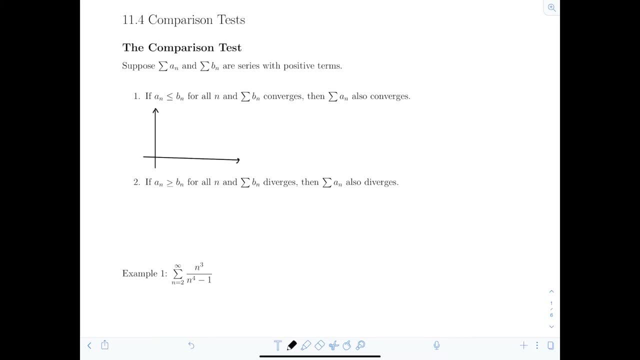 So here I'm going to just give an example. We're going to plot some of the terms a, n and b, n, and remember, we require, required that all of the terms of the series be positive, right? So I know, the x-axis, or the 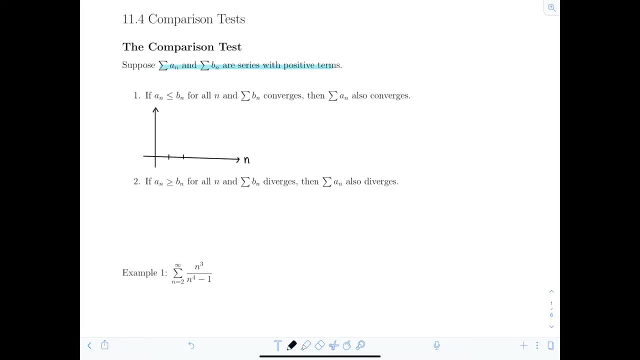 n-axis is bounding them below and I have b? n and the sum of b? n is a convergent series. So say this is b 1,, this is b 2, so I know for sure the terms are decreasing right: b 4,, b 5, and then a n. 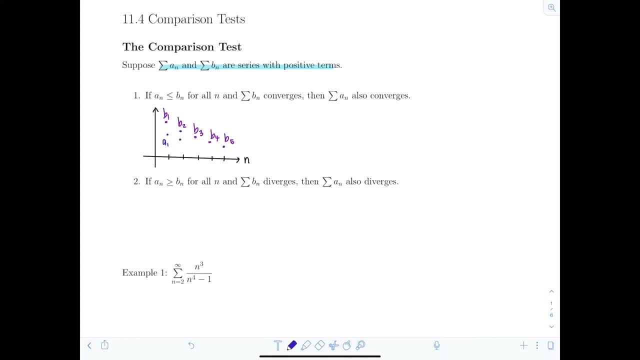 is less than or equal to b n for all n. So here's a 1, a 2, a 3, a 4, a 5.. So clearly, if I know that the series with larger terms converges, and I'm comparing it to: 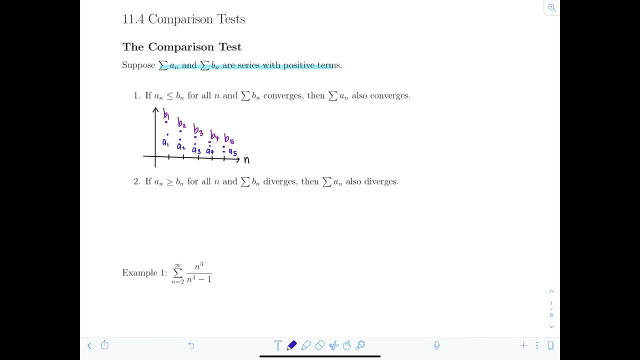 another series whose terms are smaller, then clearly this sum, the sum of a? n, must also converge, okay. Second statement of the comparison test: If a? n is greater than or equal to b? n, for all n and the sum of b? n diverges, then the sum of a? n diverges also. So I'm going to give you an example: what 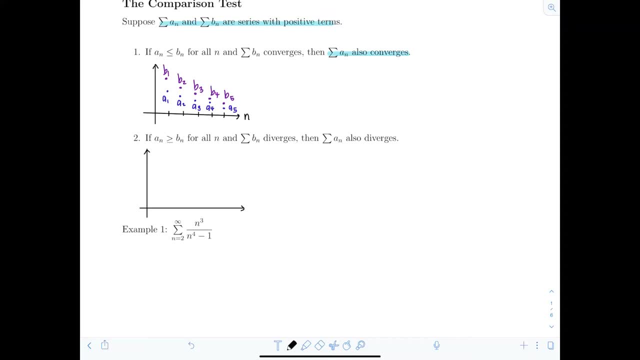 this looks like. So here's n, and then we're going to plot maybe a few terms for b, n, b1,, b2,, b3, I should put one more right here: b4,, and that sum diverges, right? Well? 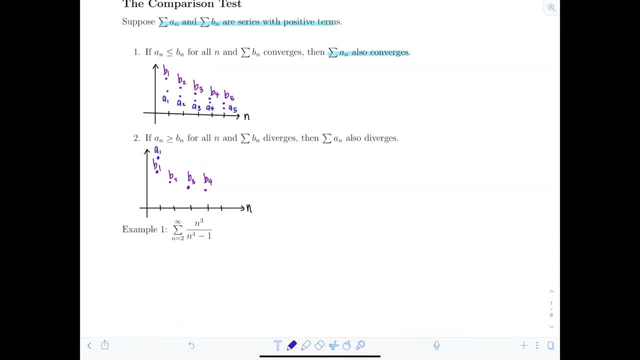 a? n is greater than or equal to b? n for all n. So here's a 1, here's a 2, here's a 3, here's a 4, etc. If I know that the sum of these smaller terms diverges, then for sure the sum of 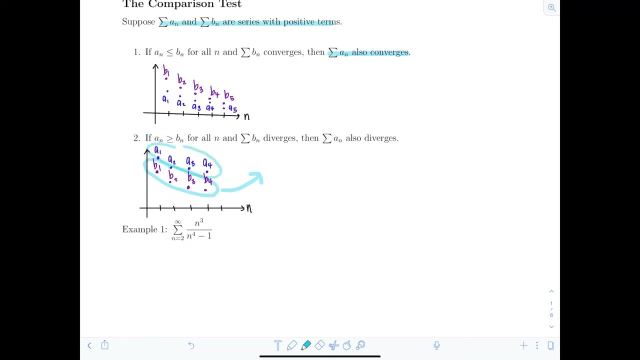 the terms of a series that are larger is going to diverge as well. okay, Now you have to be really careful when using the direct comparison test, because there are two other scenarios in which you have no information. So, looking here at the first case, 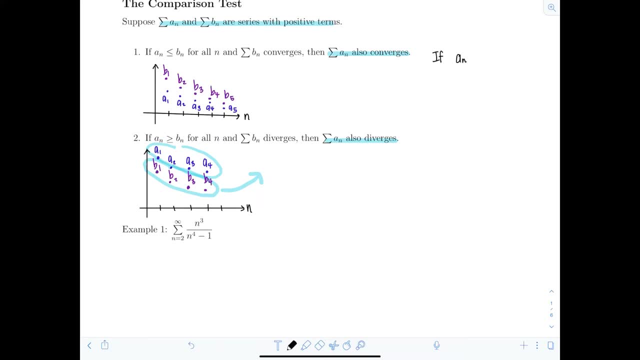 if you're able to say that the terms a, n are less than or equal to b? n, for all n and the sum of b? n diverges, then you have no information. It's inconclusive because the sum of a? n could converge or diverge, right. So the only way that you can say for sure: 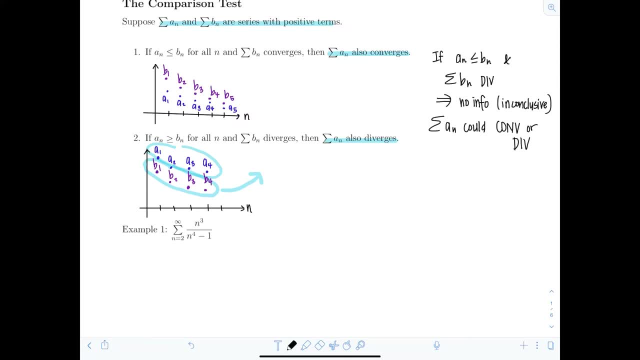 the sum of a? n diverges is if you have no information. So the only way that you can say the sum of a? n converges is if you know the sum of b? n converges. That way, it basically forces the sum of a? n to converge as well, and that's why we require the terms to be positive. 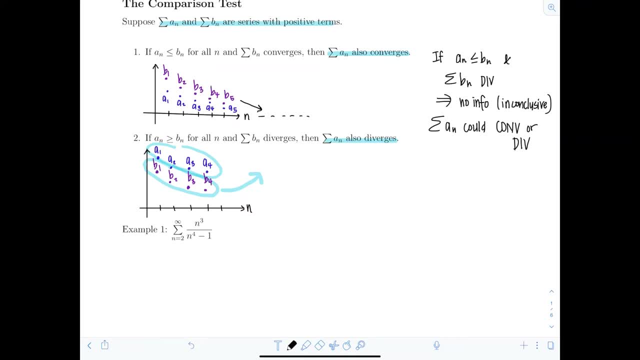 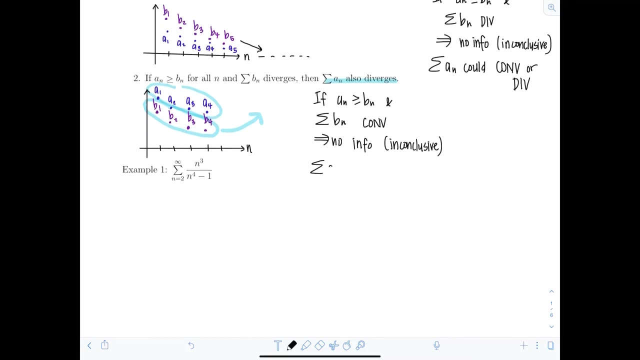 so it serves as a lower bound. Similarly, if you know that a? n is greater than or equal to b? n and the sum of b? n converges, no info. This is again inconclusive. The sum of a? n could also converge or diverge. Basically, you're saying: 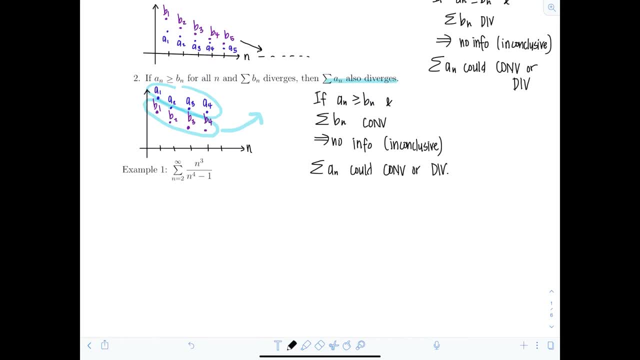 oh, I have a series. it converges. and then here let's look at another series whose terms are larger. They could converge too, or they could just blow up and go to infinity. So who's to say? So make sure you memorize and understand the comparison test very carefully. 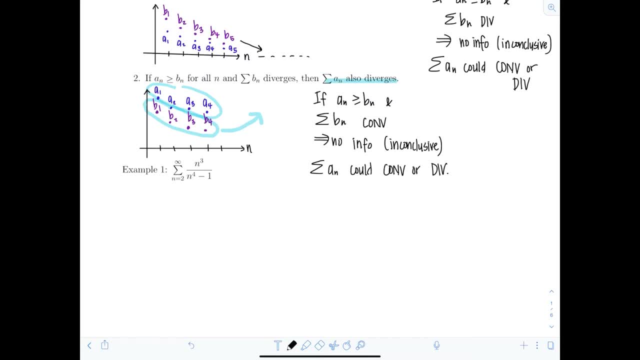 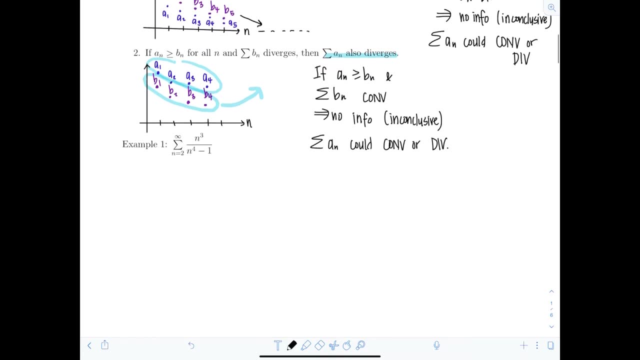 So that you don't misapply it. Okay, let's look at an example. here We have the sum n equals 2 to infinity of n, cubed over n to the fourth minus 1.. Now notice, the index starts at 2, so we're. 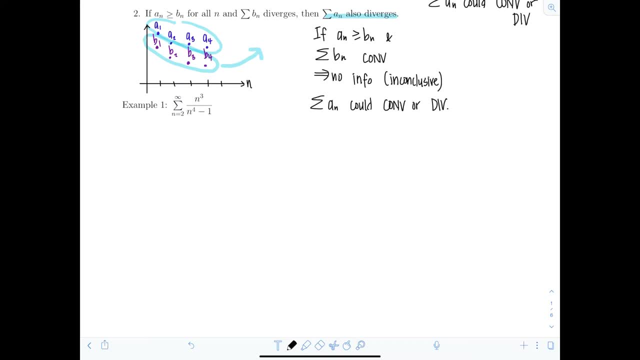 going to have to be very precise throughout our notation. If we started at 1, then the first term would not be defined. So the terms here of the series a, n are n, cubed over n to the fourth minus 1.. 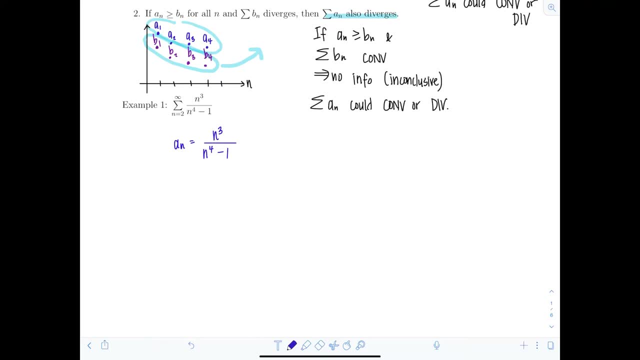 Now, whenever you're going to apply the comparison test, you already have to have an idea or a feeling as to what the series is going to do. That way, you can choose b? n appropriately right, Because you want to, if you're going to show that it's greater than the terms of some other series. 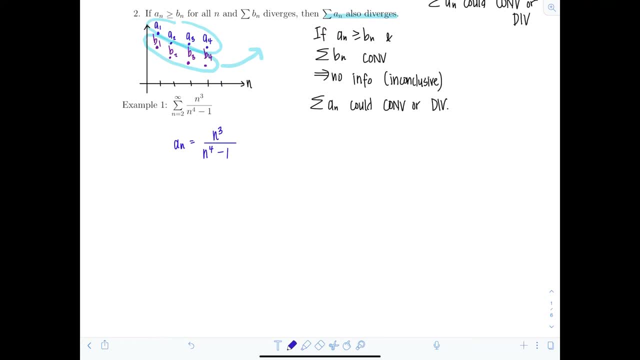 then that means you're already suspecting that it's going to diverge. Or if you're trying to show that your terms are smaller than the terms of another series, that's because you suspect it's already going to converge. So you do need to have a feeling as to what this thing's doing. 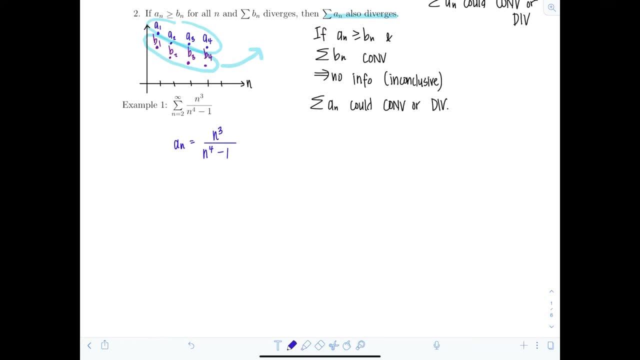 So use the exponents in the numeric equation. So you have to use the numerator and denominator to help you decide. Notice, the highest power of n: in the numerator is to the third and in the denominator it's to the fourth. So basically, 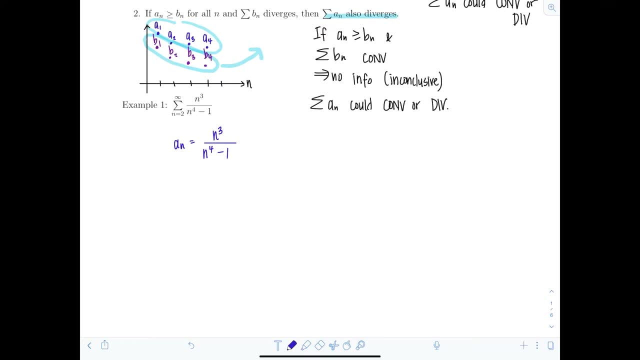 the denominator is one degree higher than the degree of the numerator. So that's reminding me of the harmonic series. So we're going to let b n equal 1 over n, right? And so now I'm going to consider the series: n equals 2 to infinity, of 1 over n. 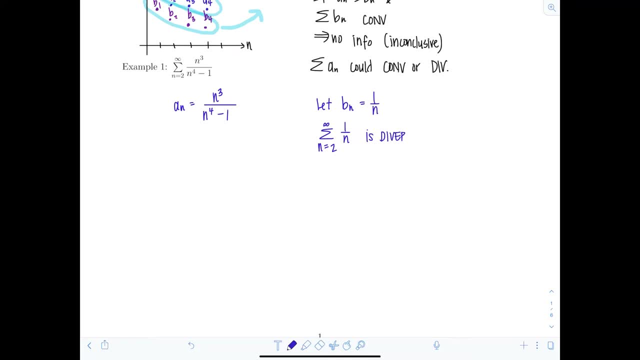 And this series, we know, is divergent because it's the harmonic series. Now, it doesn't matter that we're starting at 2 instead of 1, right? If the harmonic series diverges and I take away a term, it's still going to diverge. Or if I add in a term: 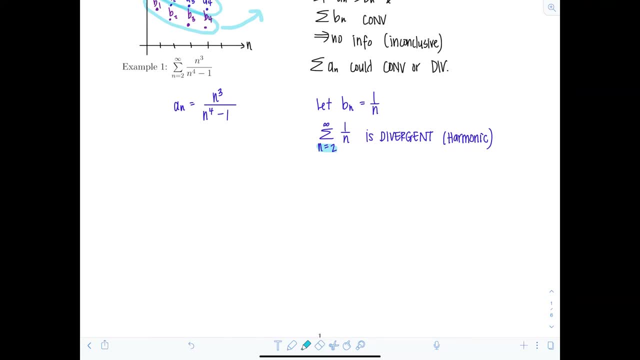 it's still going to diverge, So don't worry about that. But I have to match that index to the index of my original series, All right? So that means I'm suspecting that the sum of a- n is going to diverge, which means I need to show that the terms a- n are larger than b? n. Can I do it? 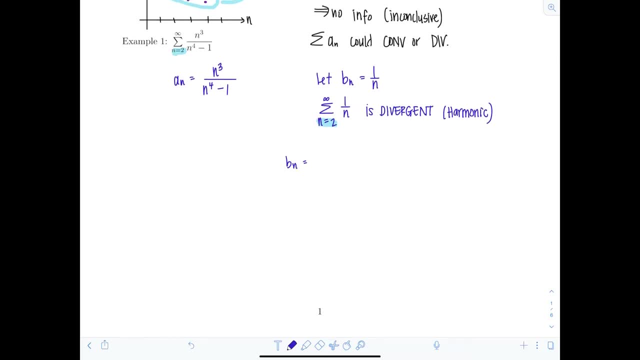 Let's see b? n, which is 1 over n. how can I make it resemble a n? Well, that would just be by multiplying by n cubed in the numerator and denominator right: n cubed over n cubed. 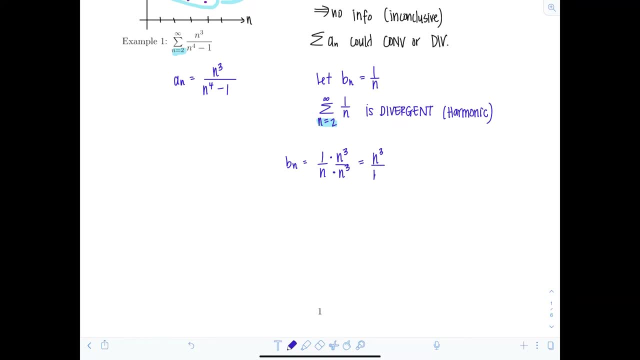 And then I have n cubed over n to the fourth. All right. Well, what's different about a n? a n is equal to n, cubed over n to the fourth minus 1.. Now what happens? Think about it If you. 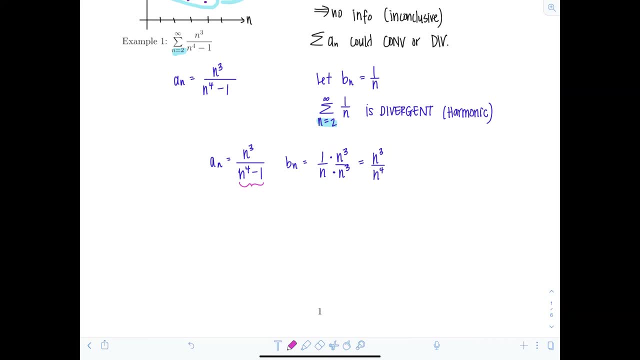 subtract 1 from the denominator. if you make the denominator of some expression smaller, you're making that overall quantity larger, right? So I'm already able to directly show that a? n is greater than b? n And that's the desired inequality, right? We know the sum of b? n diverges. 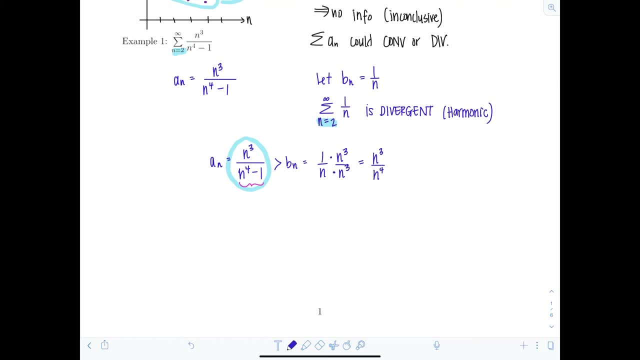 a n is larger than b? n, I can say the sum of a- n diverges as well. So now let's just write that up. So this implies that the sum- remember we're starting n- equals 2 to infinity of a- n, which 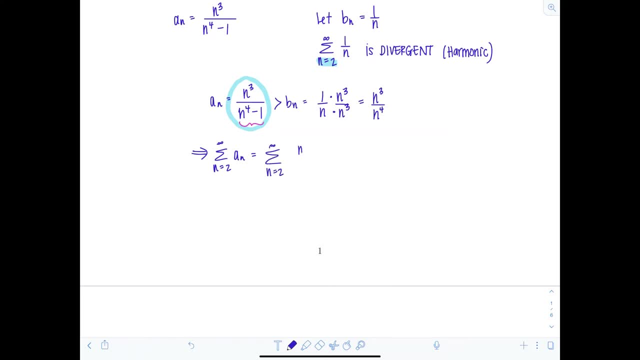 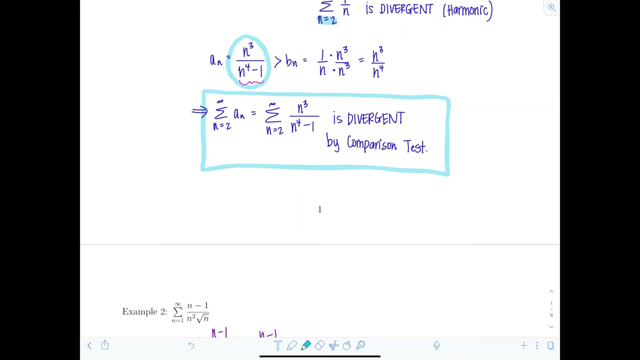 is the sum n equals 2 to infinity of n. cubed over n to the fourth, minus 1 is divergent and you have to say how you know by the comparison test. Okay, let's box this. it looks so nice. Now, make sure I'm going to recap kind of what's essential for a complete and correct answer, because 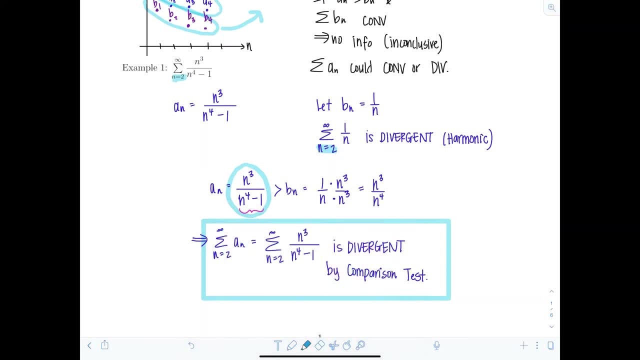 I'm sure you're wondering. So when you choose b? n, write out what it is, Make sure you have a complete and correct answer. So when you choose b? n write out what it is, Make sure you say you don't say the sequence is convergent or divergent. you write the series. 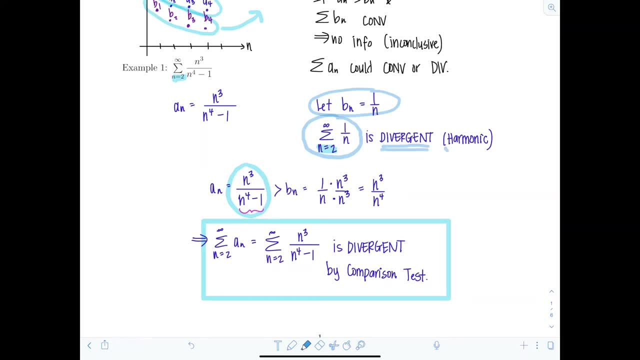 the sum of b? n is either convergent or divergent and you have to justify how you know. Either you say it's a harmonic series, you say it's a p series, you say it's a geometric series, some reason. Okay, you can't just say it's divergent or convergent and not explain yourself. 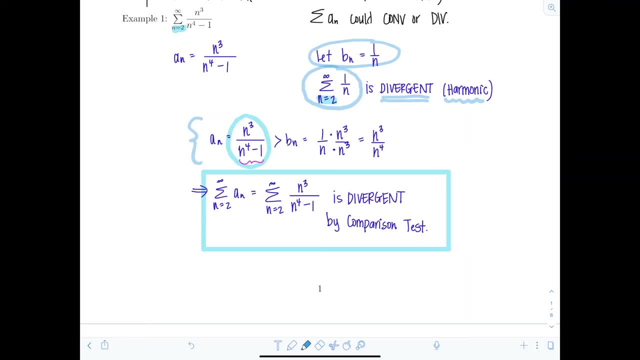 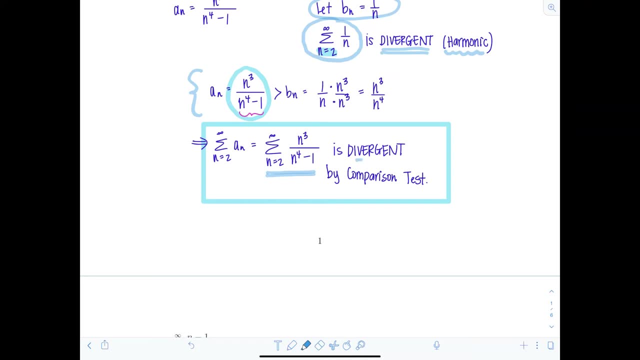 Then you have to show your inequality, the appropriate one, and then, when you write out your final statement, you need to write the original series, the sum of a- n. you have to state whether it's convergent or divergent, and then you have to state what test you used and how. 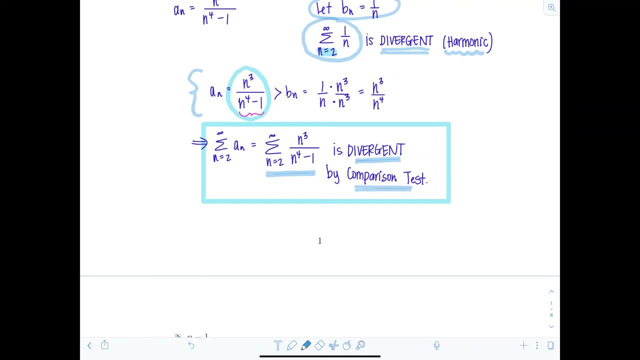 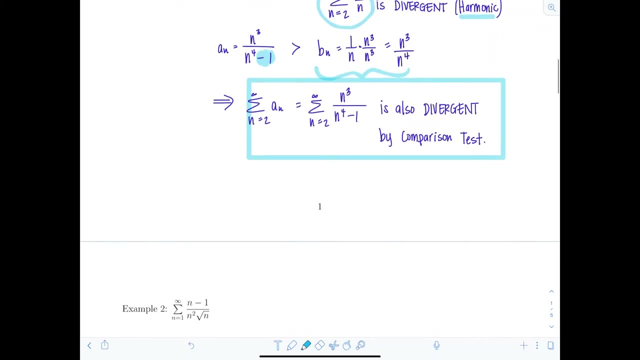 you know. Okay, so with practice, make sure you don't leave any details out. Basically, you're justifying that you understand exactly what's going on and how these series are behaving. Let's move on to another example. So here we have. the sum n equals one to infinity. 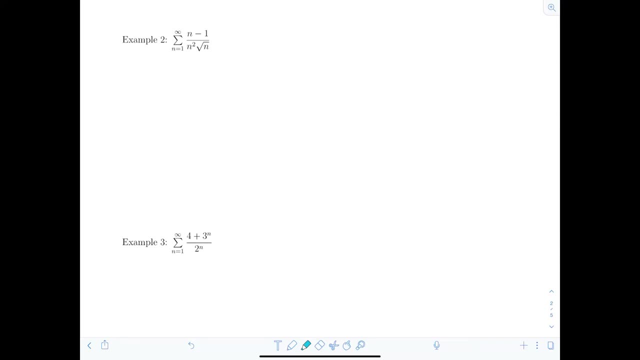 of n minus one over n squared rad n. So first let's identify what a n is, what the terms are here. So a n is n minus one over n squared rad n, and I can simplify the denominator right using my laws. 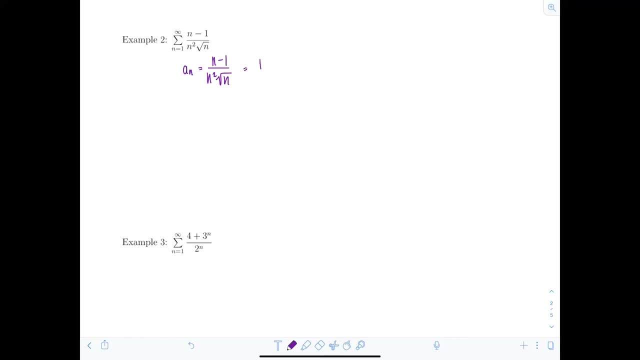 of exponents, because that's n squared times n to the one-half power. So this is n minus one over n to the five halves. Okay, so again, in order to figure out what we think b? n should be, we want to know whether b? n is growing or shrinking, however you want to think about it, and whether or not we 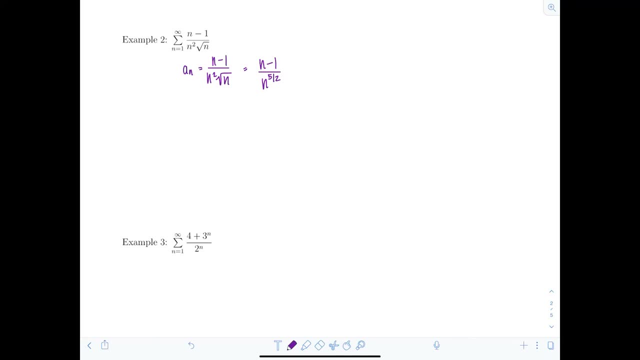 suspect it's going to converge or diverge. So notice: I have n to the first in the numerator and n to the five halves in the denominator. So if I just let b n equal n over n to the five halves, that's going to be one over n to the. if I subtract my exponents, three halves. And what do we know? 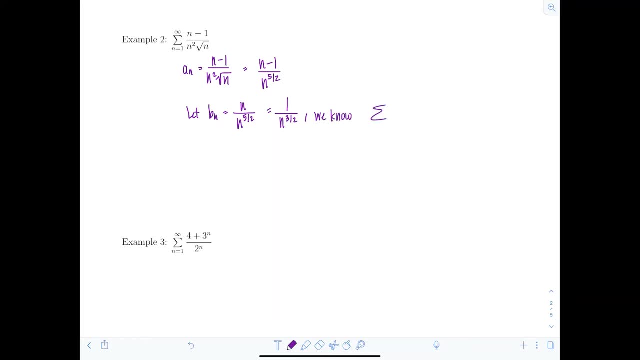 We know that the sum n equals one to infinity of one over n to the three halves does what It converges. How do I know that It's a p series? and here's my justification: p equals three halves, which is greater than one. So what does this mean? Well, we need to show. 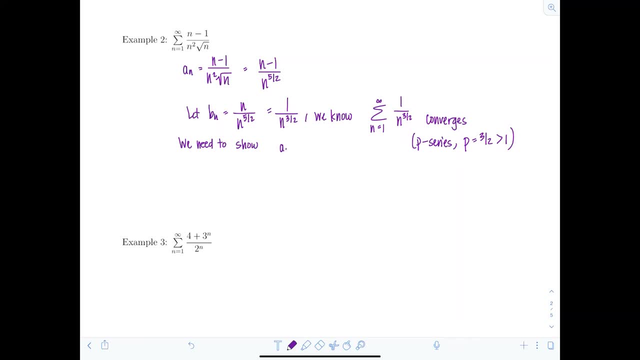 since I know b? n converges, that our terms a? n are less than or equal to b? n. Can I do it? Well, a? n is n minus one over n squared rad n, and that's definitely going to be less than if I just had. 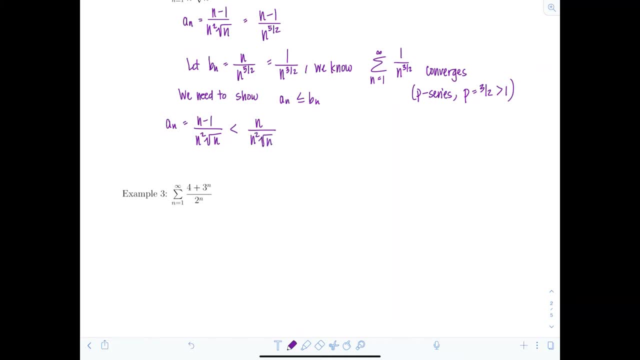 n over n. squared rad n. right, If I'm subtracting one from the numerator, then those terms are going to be smaller, And this is equal to n over n to the five halves, which is 1 over n to the 3 halves, which is bn. 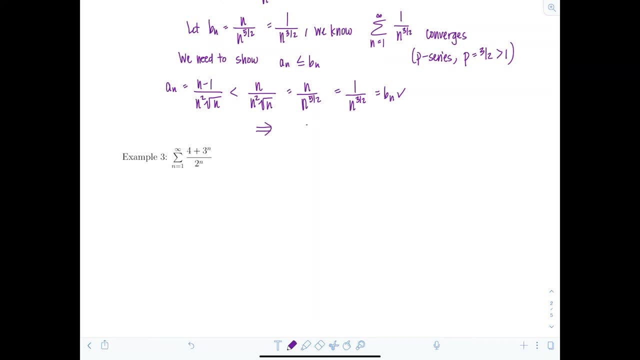 So what does this tell us? Well, this tells me that the sum n equals 1 to infinity of an, which was n minus 1 over n squared rad n also converges. How do I know? By comparison test. Okay, if I'm unable to show that the terms of my series are smaller. 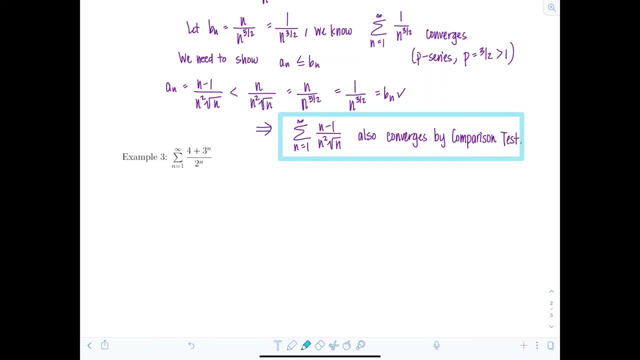 then I'm not able to use the comparison test. If they're larger, then my series could converge or diverge. I have no information, So the statement has to be very precise when using the comparison test. Okay, let's look at another one here. 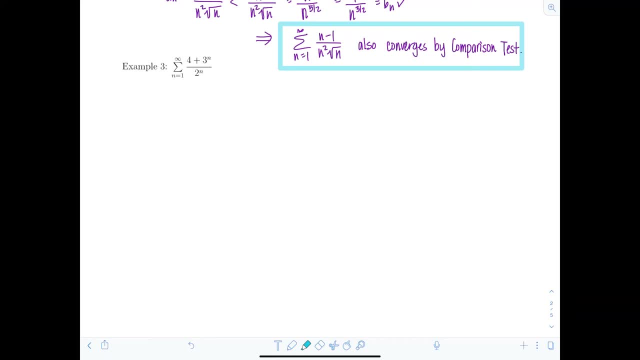 Example 3, we have the sum n equals 1 to infinity- of 4 plus 3 to the n, squared rad, n squared rad, n n over 2 to the n. All right, so an is 4 plus 3 to the n over 2 to the n. 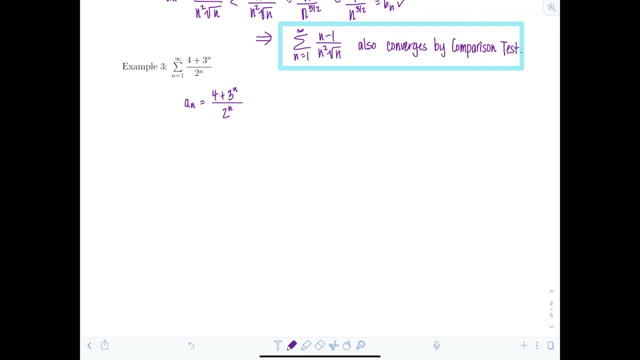 Okay, what do you want to use for b, sub n? Usually you just kind of like: strip away all the added and subtracted constants and get to the meat of the terms, So without the 4 added in the numerator right, because the constant's not going to affect the growth too much. 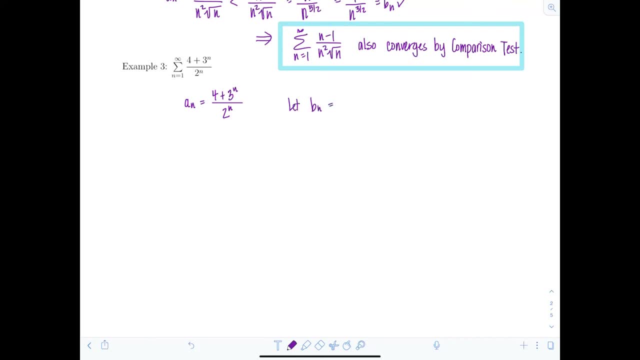 I'm just going to let b sub n be 3 to the n over 2 to the n, So that's going to be 3 over 2 to the n. Okay, does this look familiar? Are we thinking geometric? hopefully, 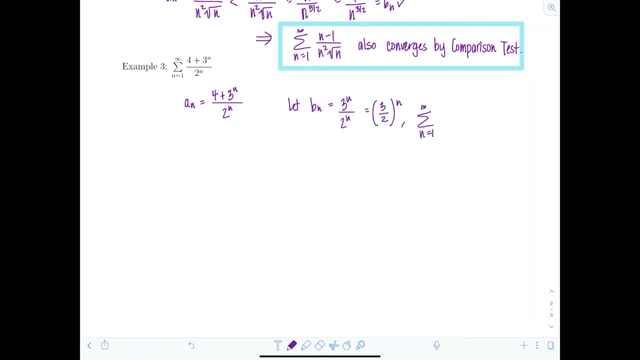 And we know the sum n equals 1 to infinity, of 3 halves to the n. What does that do? It diverges, right. How do I know it? Because it's geometric, With r equaling 3 halves, which is greater than 1, right. 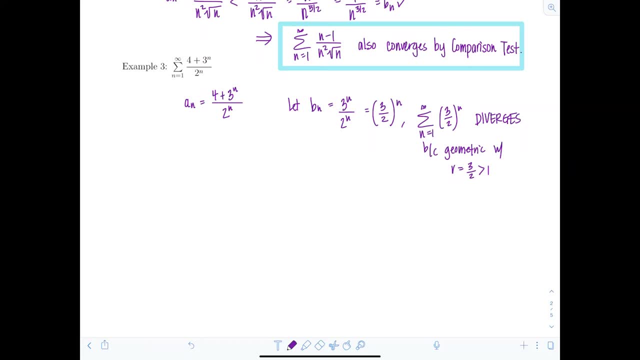 Make sure you include all of that for your justification. So okay, I have a known series. It diverges. If I'm going to use the comparison test, then I need to be able to show that the terms of our series are larger. 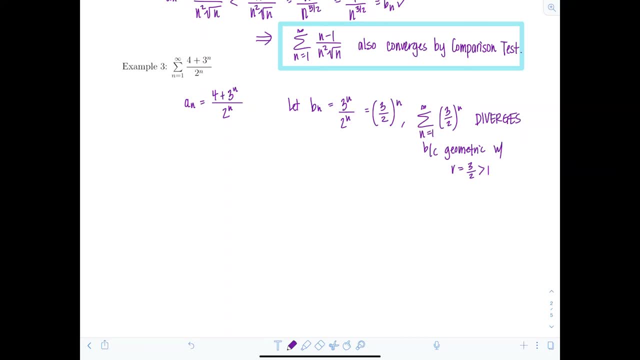 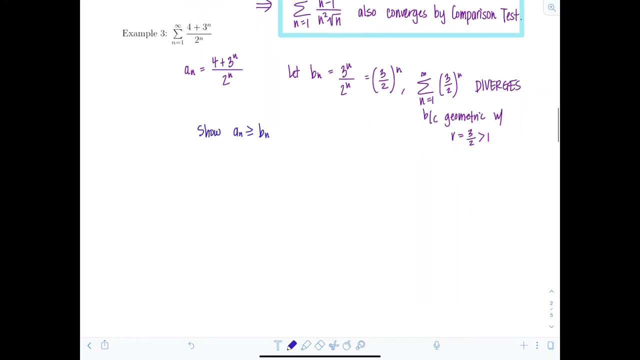 than the terms bn, in order to say that our series diverges as well. Okay, here I do it. So I need to show that an is greater than or equal to bn. All right, let's see. So an is 4 plus 3 to the n, over 2 to the n. 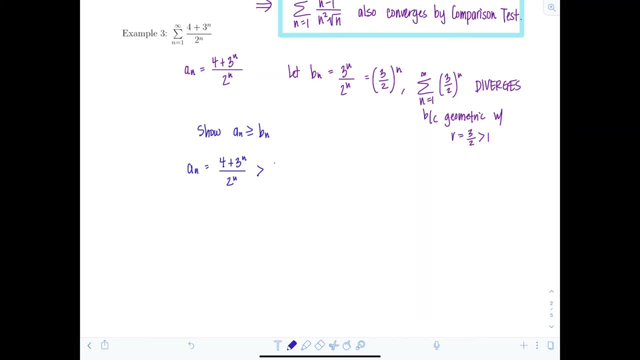 Well, if I get rid of the 4, right, Isn't this greater than 3 to the n over 2 to the n? If you add 4, the whole term becomes larger. The quantity becomes larger, And this is 3 over 2 to the n. 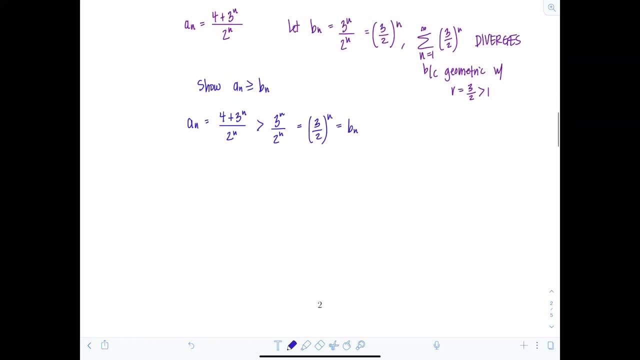 Which is b sub n. Great, that one wasn't too crazy. So this means the sum n equals 1 to infinity of an, which is the sum n equals 1 to infinity of 4 plus 3 to the n over 2 to the n. 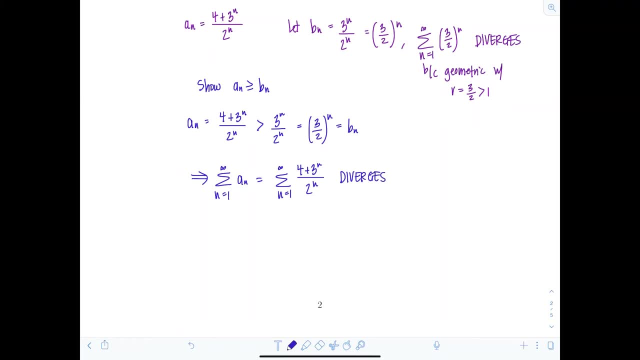 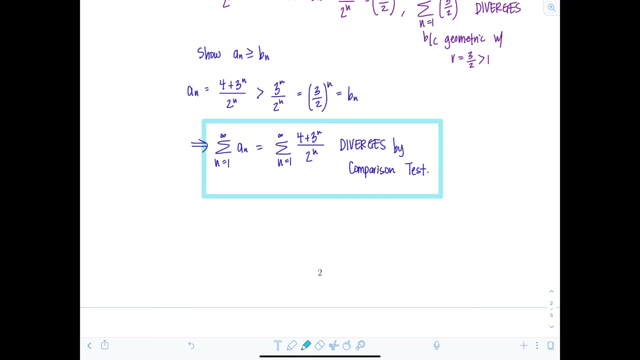 also diverges by the comparison test. All right, Nice job. Okay, example 4,. we have: the sum n equals 0 to infinity of 1, plus sine n over 10 to the n. So to get started, let's list out what an is. 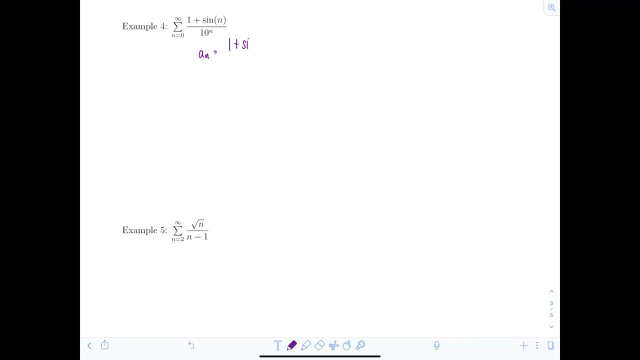 So an is 1 plus sine of n over 10 to the n. And remember, before we choose bn, we kind of want to, we want to get a feel for what we think is going to happen here with this series. Well, there's 1 plus sine n in the numerator. 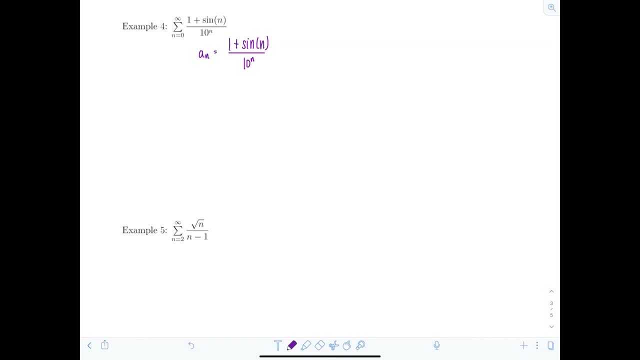 I know sine oscillates, but it's bounded right, It's bounded between negative 1 and 1.. So really, what's controlling the growth of the term? is that 10 to the n in the denominator, 10 to the n? that means this is geometric right. 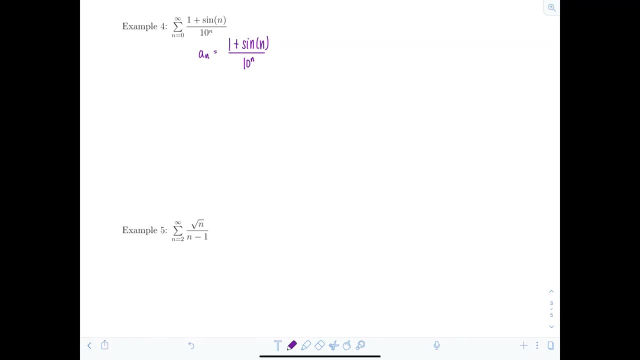 And so r would be smaller than 1. And it looks like this most likely will converge. So if I'm trying to show that this series is going to converge using the comparison test, I want to show that it's smaller right than some other convergent series. So can I come up with an upper bound for my terms? a, n. 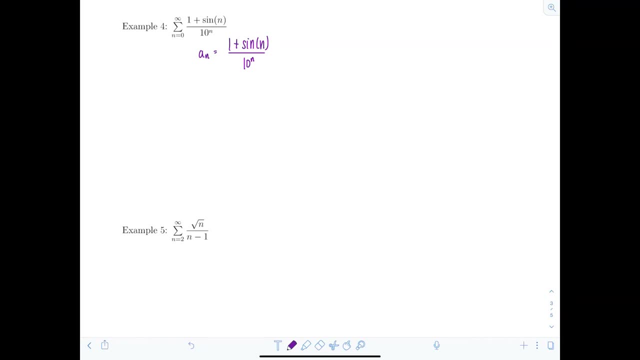 Well, to start, we're going to do this one a little bit backwards. I'm going to bound it and then talk about what b? n is. So I choose b? n appropriately. I know sine n, I can bound right, Sine n, I can bound by 1 and negative 1.. And then I'm going to try to make this match a? n. 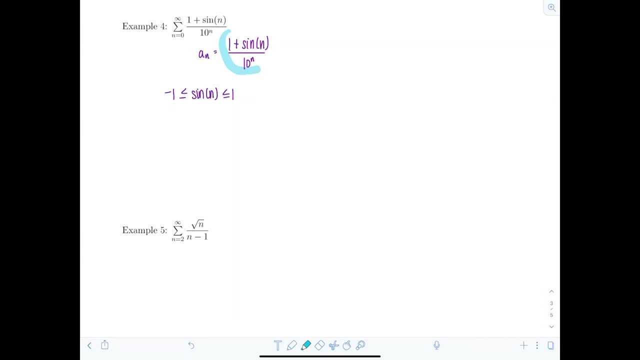 I want to make it match this expression in the middle. So what would I need to do? Well, let's go through and add 1 across our inequality. So now I have: 0 is less than or equal to 1, plus sine of n is less than or equal to 2.. 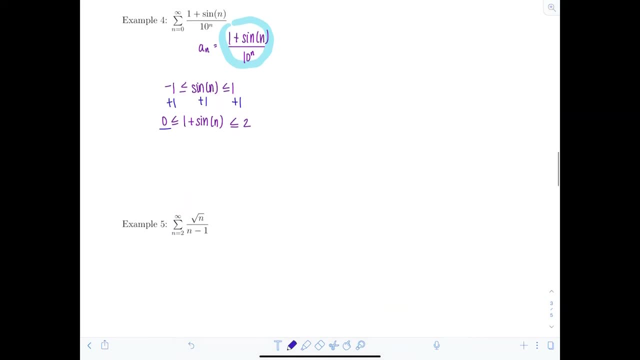 And then, last thing, I'm going to divide through by 10 to the n. I know that's never 0, so it's okay to divide through by it And it's not negative. Okay, So now we have: 0 is less than or equal to 1, plus sine of n over 10 to the n, which is our an right. 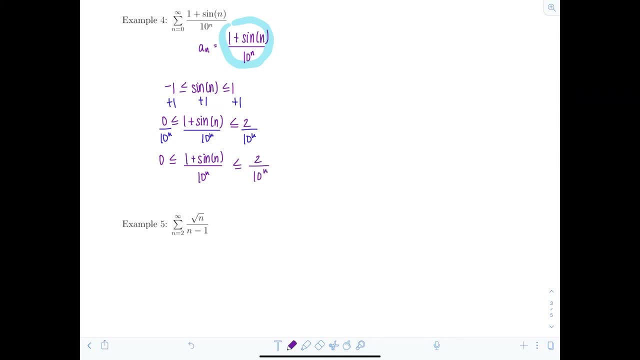 Which is less than or equal to 2 over 10 to the n. So notice here this is an- and I found an upper bound for it already- 2 over 10 to the n. So how about we let that be bn. 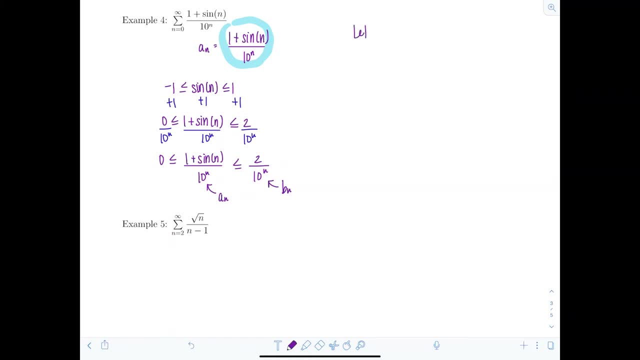 Can we say something about it? Well, let's see, let bn equal 2 over 10 to the n, Then I know the sum n equals 0 to infinity. 2 over 10 to the n, that's the same as 2 times 1. 10th to the n- right. 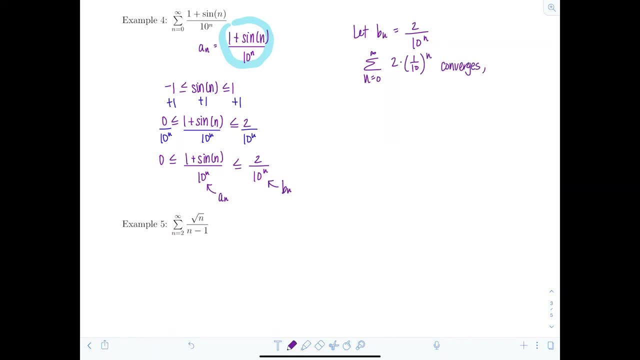 And that converges? why? Because it's geometric r is 1- 10th, Which is less than 1.. Again, when you're justifying the convergence here, just saying it converges, it's geometric is not enough. 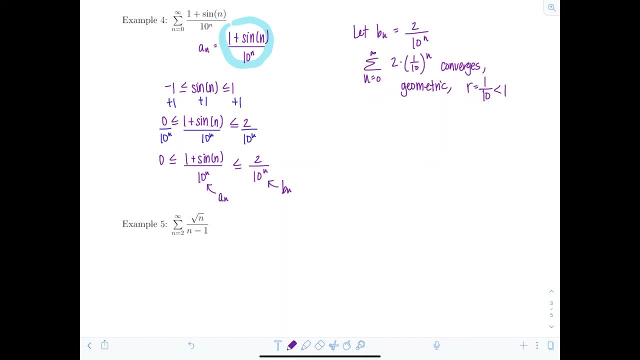 You need to prove that you know why, that you identify r and the fact that it's less than 1.. You have to show that you understand the statements behind all of these things. Okay, so, since we've already shown, remember this one. we did a little bit different order. we already showed our inequality. 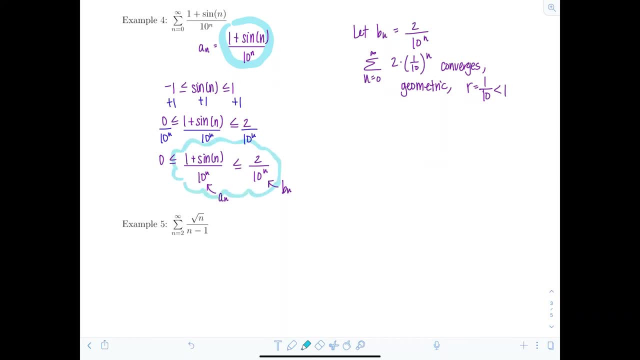 I know my terms: an are less than bn, Then I'm basically, I'm basically done right. So, since we showed that an, which is 1 plus sine of n over 10 to the n, is less than or equal to bn, which is 2 over 10 to the n, 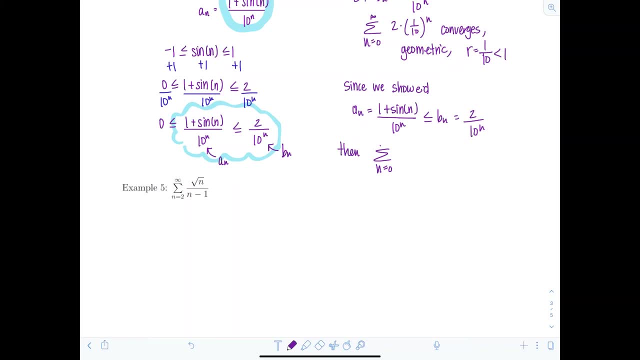 Then the sum n equals 0 to infinity of an, which is the sum n equals 0 to infinity of 1, plus sine of n over 10 to the n also converges. what am I missing? Yep, by the comparison test. 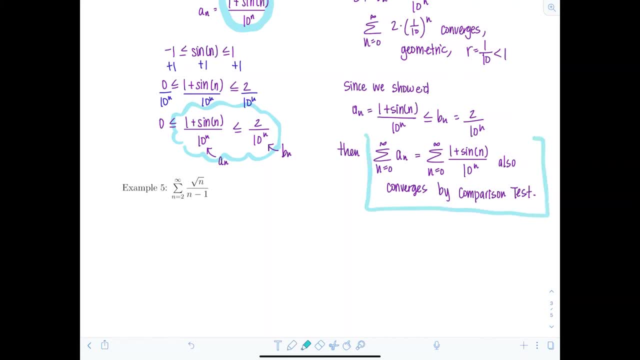 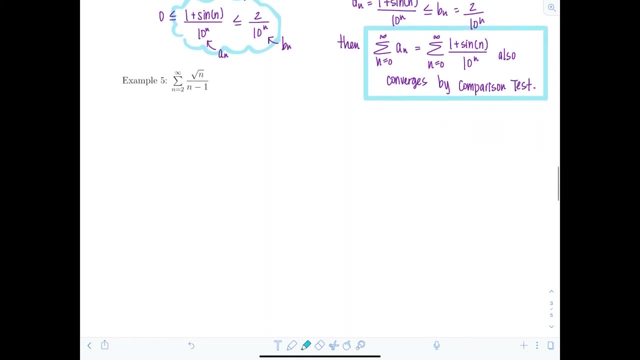 Okay, let's box that part Beautiful. One last one here. So we have the sum n equals 2 to infinity notice our index is starting at 2 again of rad n over n minus 1.. Okay, so an is rad n over n minus 1.. 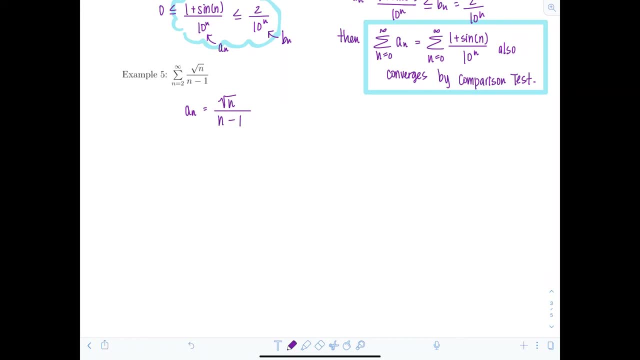 What do you suspect? Is it going to converge or diverge? What do you think? So I see rad n is the highest power of n in the numerator. so that's n to the 1 half, and then I have n minus 1.. 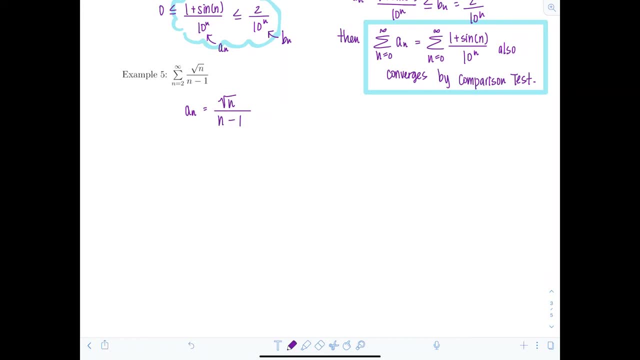 So n to the first is the highest power in the denominator, So that's growing approximately as fast as 1 over rad n, right? So let bn equal 1 over rad n. and what do we know about the sum- Notice I'm going to have to start at 2 to infinity- of 1 over rad n. 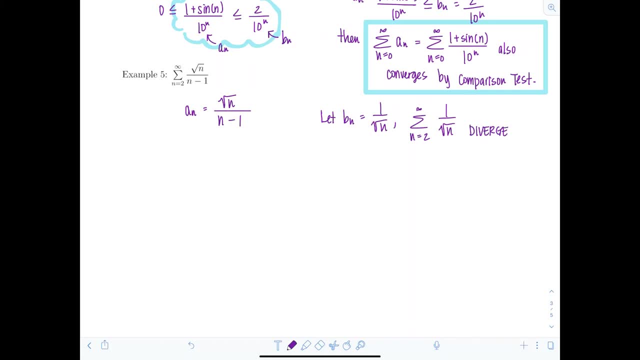 Well, that diverges Because it's a p-series with p equaling 1 half, which is less than 1.. So I need to show that an is greater than or equal to bn. right, If I'm comparing the terms of my series to the terms of another known series, that diverges. 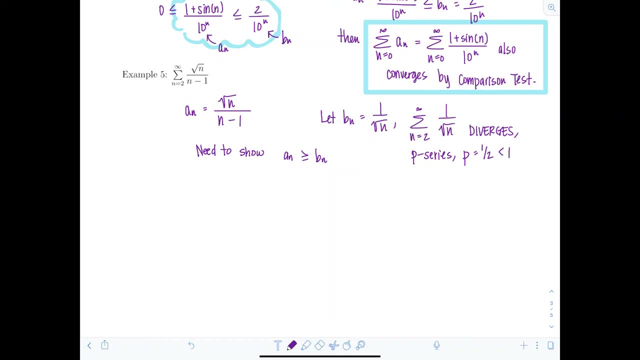 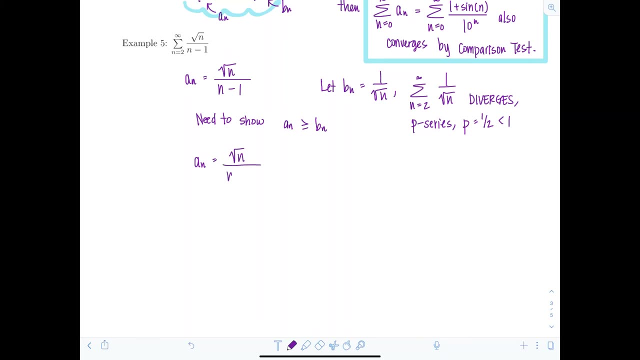 I better be able to show that my terms are larger. Can we do it? Well, let's see here. So if an is rad n over n minus 1, and I added 1 to the denominator right, That would make the new denominator smaller. 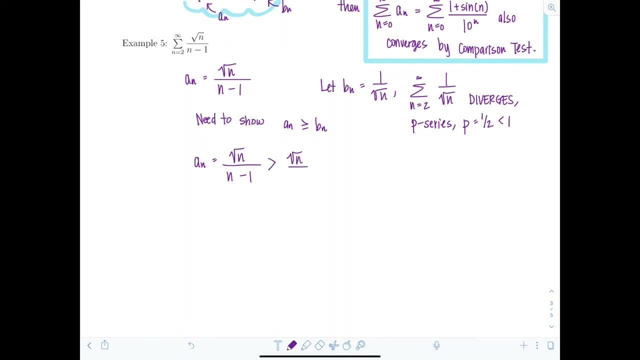 So this would be greater than just rad n over n. Think about it: If I add 1,, that's bigger. So this whole expression is now smaller, And rad n over n, that's the same thing as 1 over rad n, which is bn. 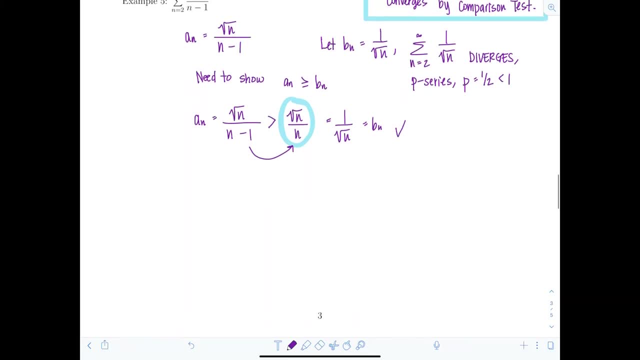 So I showed the proper inequality. So this implies that the sum n equals 2 to infinity of an, which is the sum n equals 2 to infinity of rad n over n minus 1, diverges by the comparison test. So we have 1 over rad n over n minus 1, which is 1 over rad n. 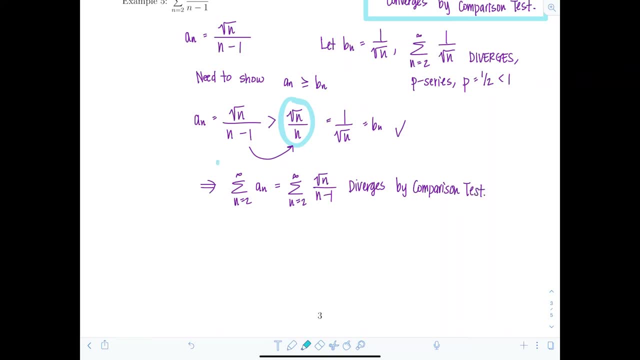 So the answer is 1 over rad n minus 1.. So that's a very good point. OK, How was that one? Now, as you can see, it can be tricky to show the inequality in the correct direction sometimes, right? 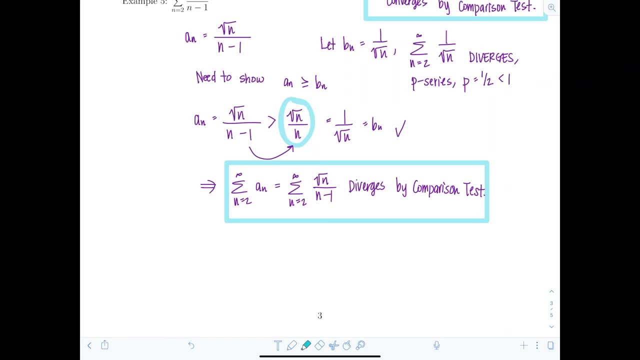 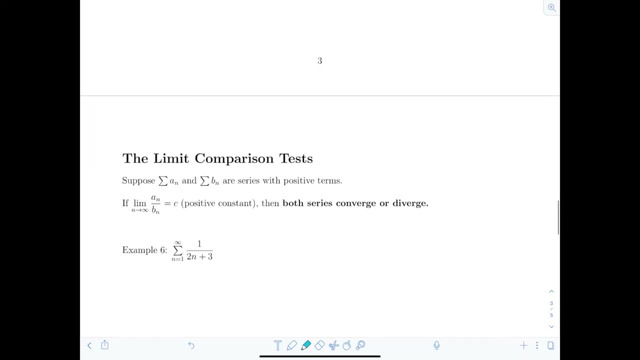 And so that's why we're going to consider another test right now, which is the limit comparison test, And this test is a lot more versatile Most of the time. I have a lot of time, I have a lot of time. I have a lot of time. 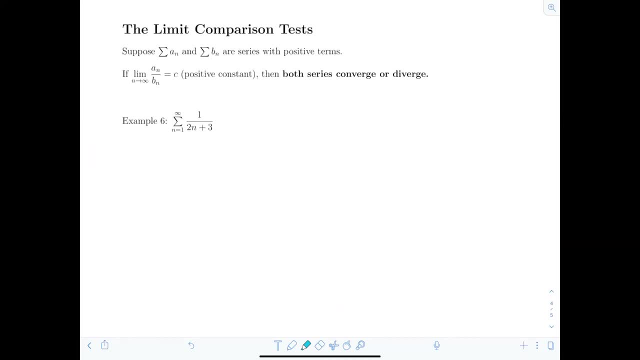 I opt for this one as opposed to direct comparison, just because you can get a statement out of it more easily. So here's what it says. Suppose the sum of an and the sum of bn. those are both series with positive terms. So same assumptions as just regular comparison test. If the limit as n 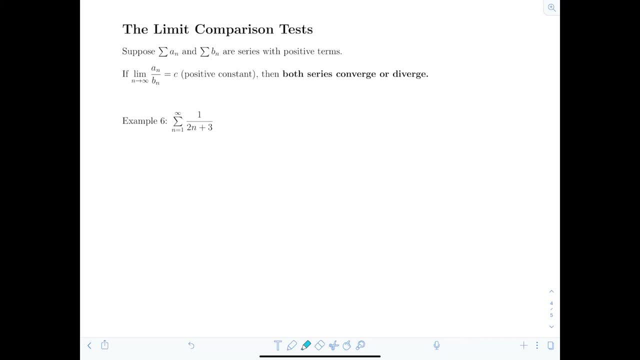 approaches infinity of the terms, an over bn equals c, which is a positive constant, then both series converge or both series diverge. It basically means they do the same thing. So as long as when you take the limit as n approaches infinity of the ratio of their terms is a constant, It can't. 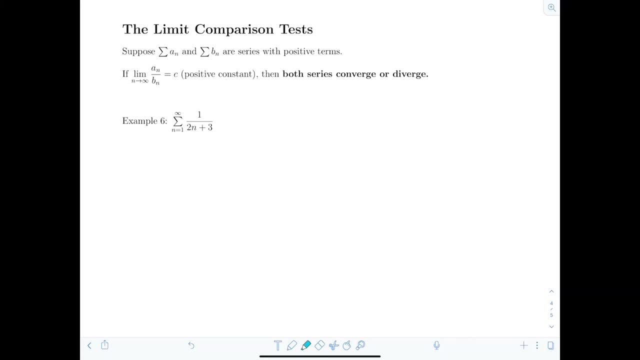 be negative, it can't be zero and it can't blow up. What does that mean? That means basically that they're growing at the same rate. right, If you get a constant, that means one isn't growing much larger or slower than the other terms, so then they're going to behave the same way. 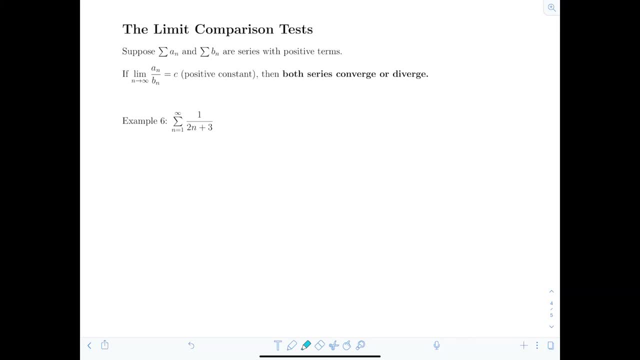 As in the fact that they either both converge or both diverge, which is nice, because then you don't have to worry about showing some sort of inequality in a particular direction. Now look here at the first example and you're going to see why you're going to love this limit comparison test. So say: 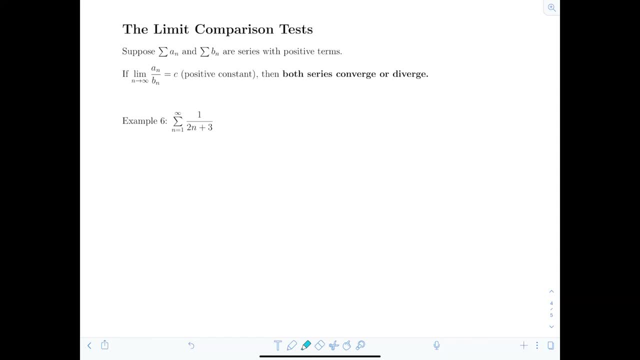 we're going to analyze the convergence or divergence of the sum. n equals 1 to infinity of 1 over 2n plus 3.. Okay, so an is 1 over 2n Plus 3.. Do you have a suspicion as to what this series is going to do? Well, look at how fast it's. 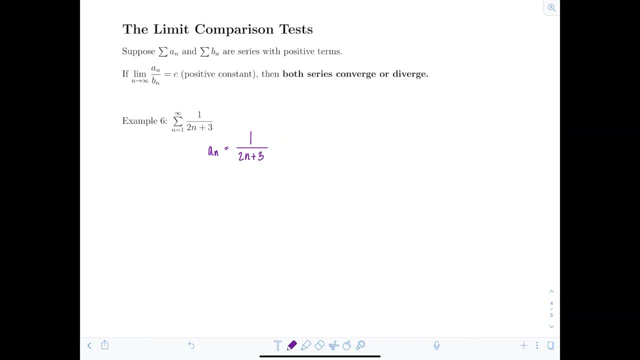 growing. Look at the terms. It's basically reminding us of the harmonic series, right, Because the numerator is the constant and then we just have n to the first power in the denominator. So let's go ahead. I'm going to let bn. 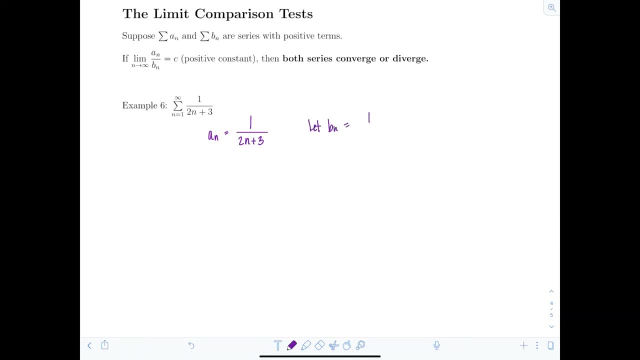 be 1 over. just to keep things easy in terms of the limit, I'm going to use 2n. If you used 1 over n, that would work just fine too. okay, And what do we know about? the sum n equals 1 to infinity of bn. Well that's, the sum n equals 1 to infinity of 1 over 2n. 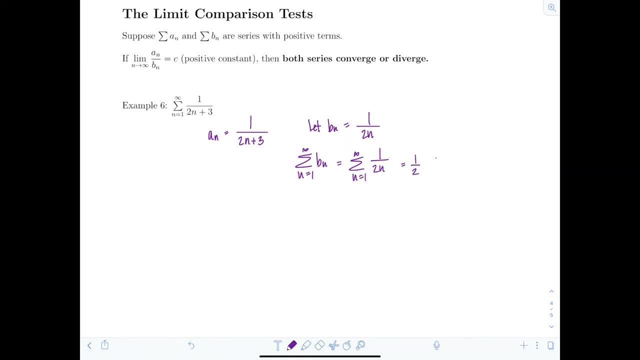 I can take that one half outside right, It's not going to make a difference, And this is harmonic And it diverges. okay, Now, before we proceed, I just want to point out something super important. So if I was using just the regular comparison test before, I would need to show 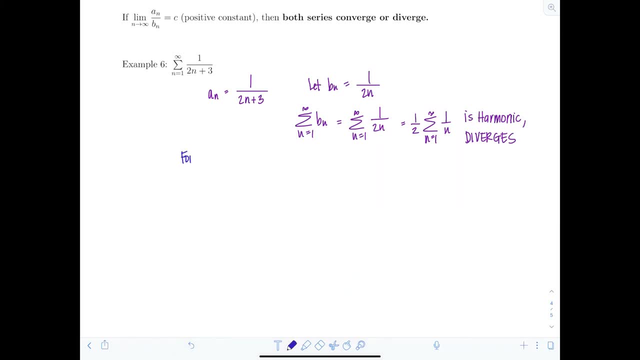 so for the regular comparison test, not limit comparison test. so for comparison test I would need to show that an is greater than or equal to bn. right, If I'm comparing it to some known series that diverges, I have to show that the terms are larger. But can I do that? Well, an is 1 over. 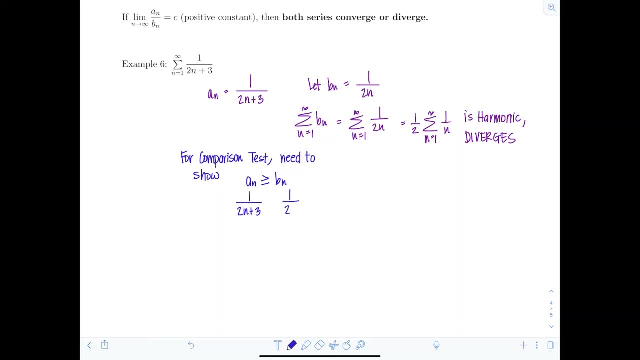 2n plus 3, and bn is 1 over 2n. I can't do it right, Because if I add 3, I'm actually making the denominator smaller. So I'm going to have to show that the terms are larger And I'm going to. 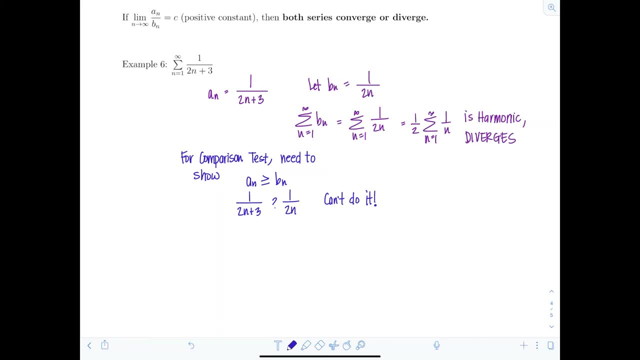 show that the terms are smaller. Does that mean, then, that this series converges? No way, Adding 3 isn't going to change it and make it shrink fast enough for it to converge. It's still going to diverge. It just means the comparison test won't help me answer the question as to whether it. 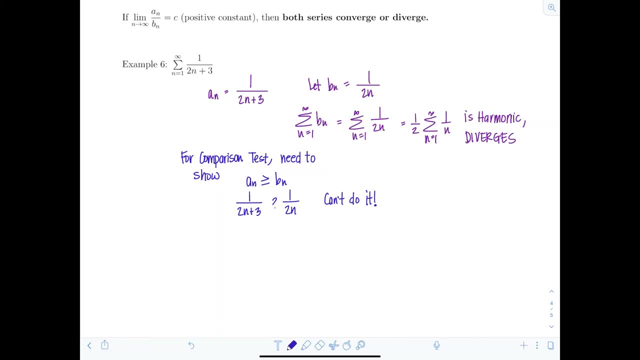 converges or diverges. So that's why limit comparison is a really strong test, because we're going to be able to get a result right now. okay, So for the limit comparison test, I'm going to take the limit of the ratio of the terms, as n goes to infinity. So I'm going to look. 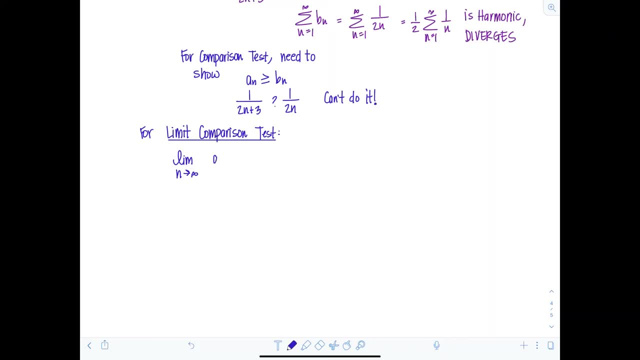 at the limit, as n approaches infinity, of an over bn. So we have the limit as n approaches infinity. an was 1 over 2n plus 3, and bn is 1 over 2n. Okay, So here I'm going to have the limit. 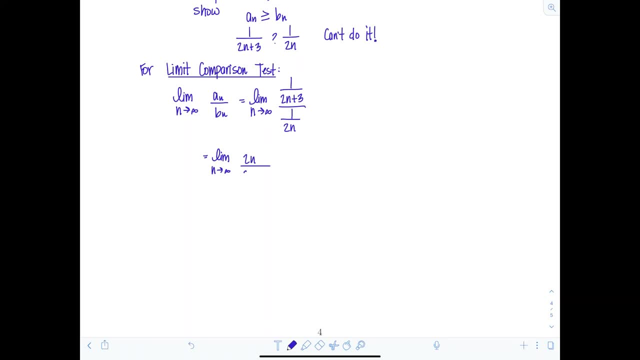 approaches infinity of 2n over 2n plus 3.. And then I'm going to multiply numerator and denominator by the highest power of n in the denominator. Well, I'm dividing by it right, Multiply by 1 over n. So then we have the limit as n approaches infinity of 2 over 2 plus 3 over n And as n 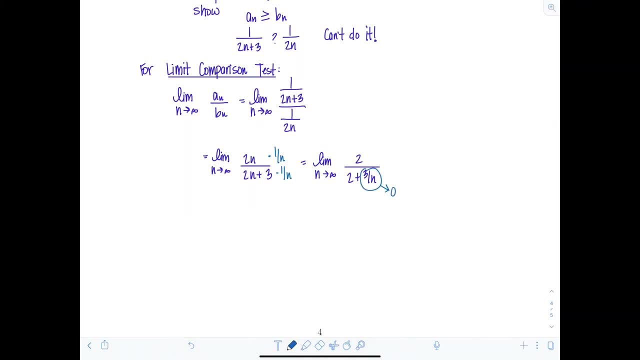 approaches infinity. 3 over n is going to go to 0.. I have 2 over 2.. Those are constants. So this limit is 1.. This limit is positive. It's a constant. Therefore, I'm able to state using: 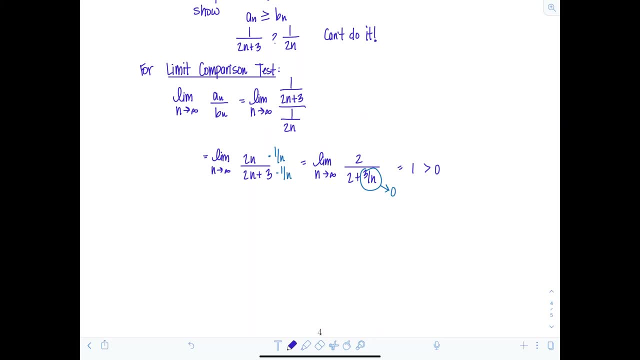 the limit comparison. I'm able to state, using the limit comparison. I'm able to state using the limit comparison test, that both series do the same thing, They behave the same way. So, since I compared it to a multiple of the harmonic series which diverges, this means: 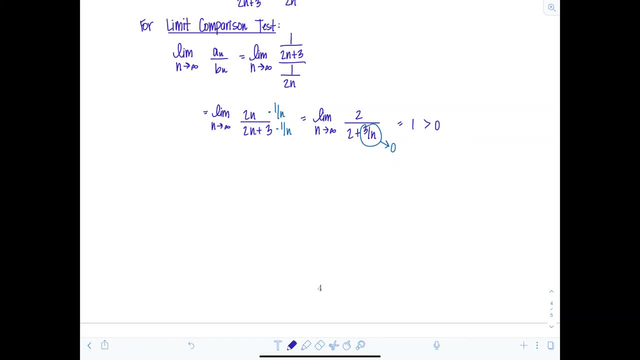 I'm going to make that look nice. You know what I mean. Everything has to look nice. Okay, The sum n equals 1 to infinity of an, which is the sum n equals 1 to infinity of 1 over 2n plus 3.. 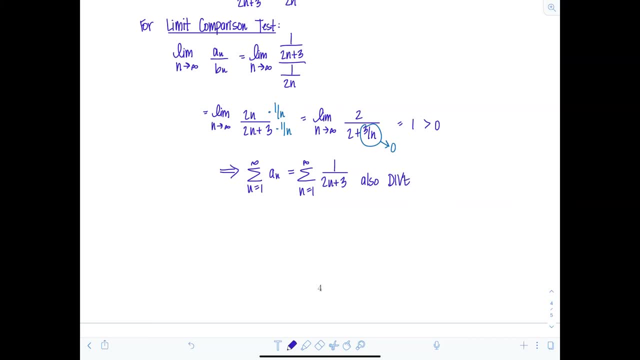 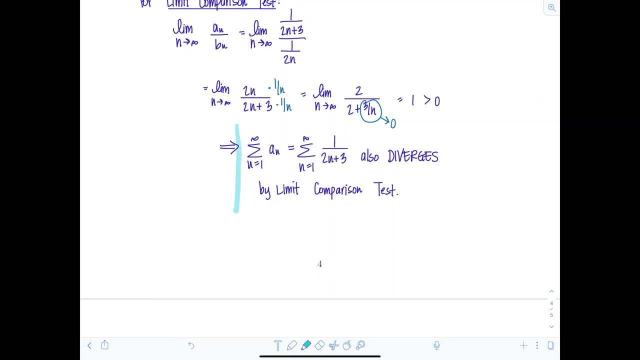 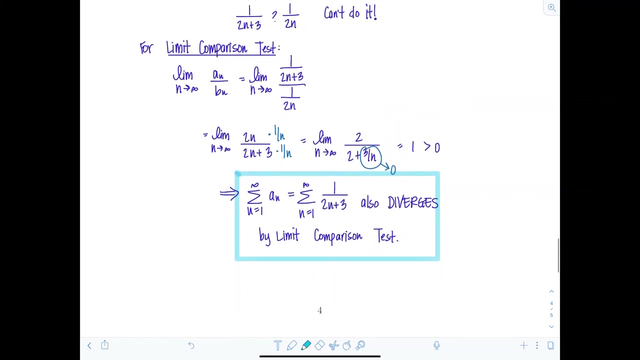 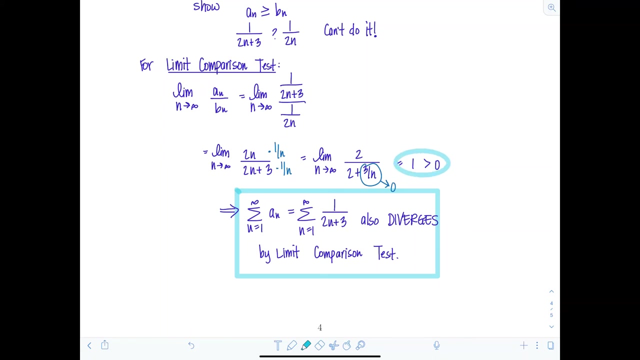 Also diverges by the limit comparison test. All right, Good. I want to point out when you take the limit- hmm, When you take the limit here, you need to show that it satisfies the condition. So you need to state that it's greater than 0, that it's not negative and that you know it's a constant. It's. 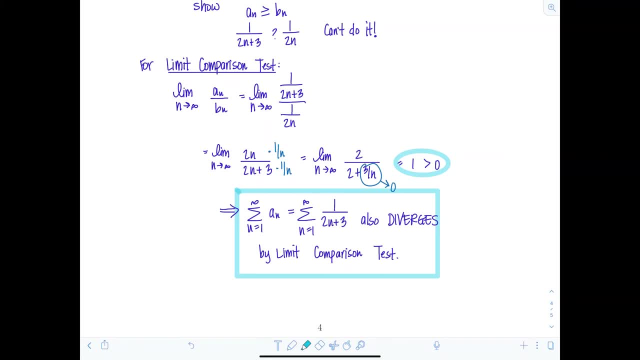 not infinity. If you got infinity or if you got 0 for the result from your limit comparison test, then the test is inconclusive. You either chose something that was not helpful for bn, so start over, or pick a different test. Also, I wanted to point out what if you had just let bn 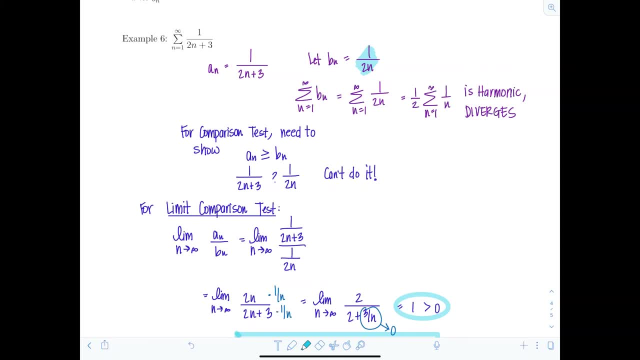 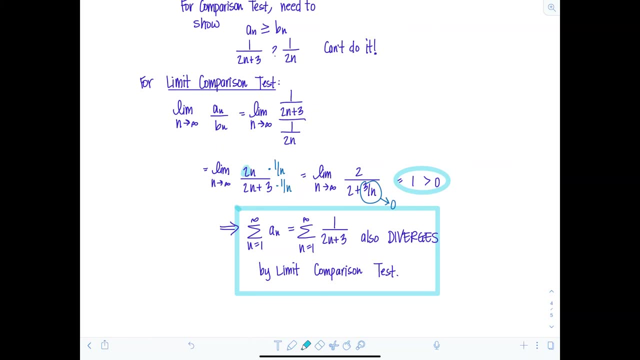 be 1 over n, not 1 over 2n. Not a problem, Let's track where that would come to play. You would have just an n here instead of 2n, right? So then you would just have a 1.. 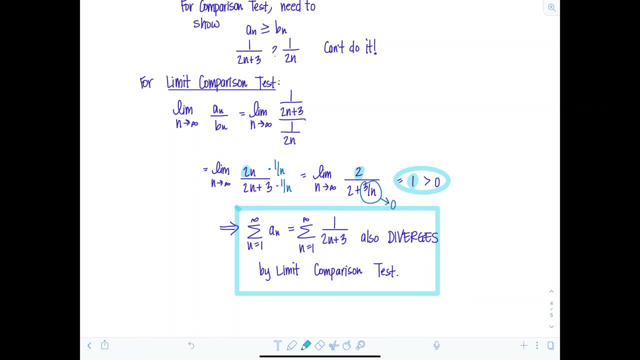 So then this would have been 1 half, But that works great. Remember limit comparison. you just need a positive constant as the result. So you would have gotten 1 half. You would have said: that's fine, This is finite, It's not negative, We're good to go. 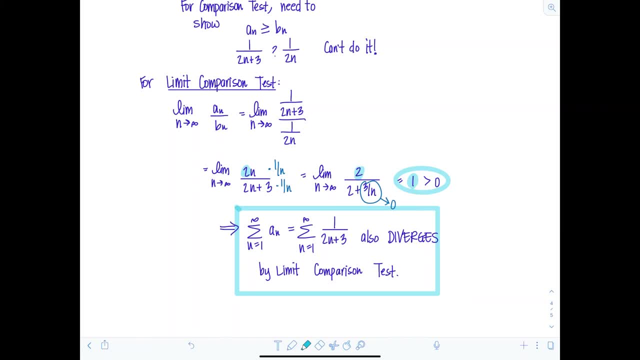 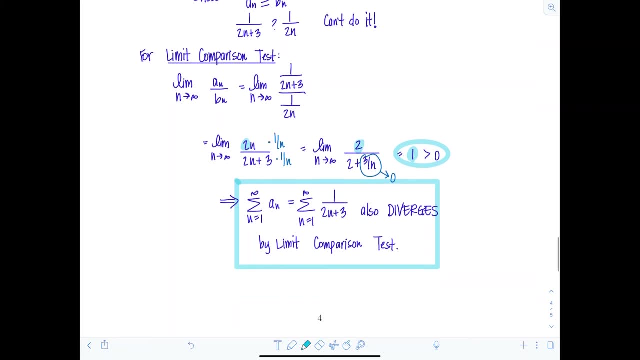 Okay, So you don't have to be so picky about your choice for bn, which is another plus to the limit comparison test over regular comparison test. Okay, One last tip, One last example, Example 7.. We have the sum n equals 3 to infinity of n plus 2 over n plus 1, cubed. 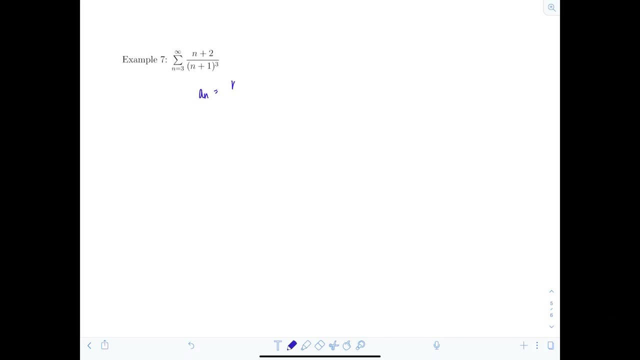 Okay, so n is n plus 2 over n plus 1 cubed. Okay, and let's choose something for bn Most of the time when the terms are looking like this, we're just going to compare it to some sort of p-series, right? 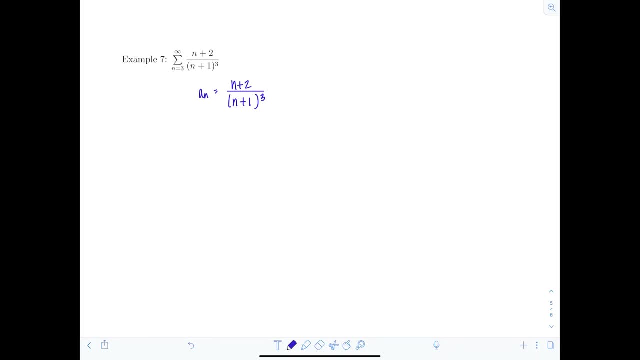 So let's see What's the highest power of n in the numerator n to the first Highest power of n in the denominator n cubed. So if I simplify that, n over n cubed, What do we get? n over n cubed. 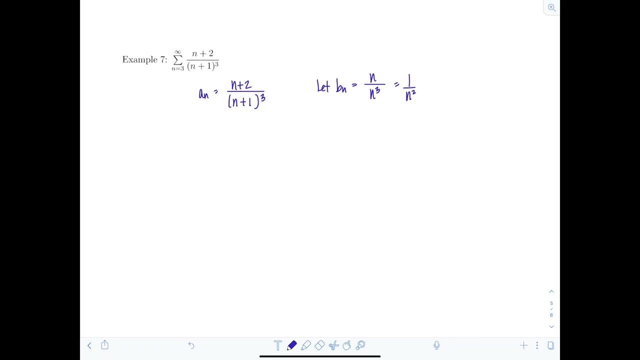 That's 1 over n, squared right. A lot of students make the mistake right here. They're going to say, oh, this is a p-series And it converges. This is not a p-series, This is just bn by itself. 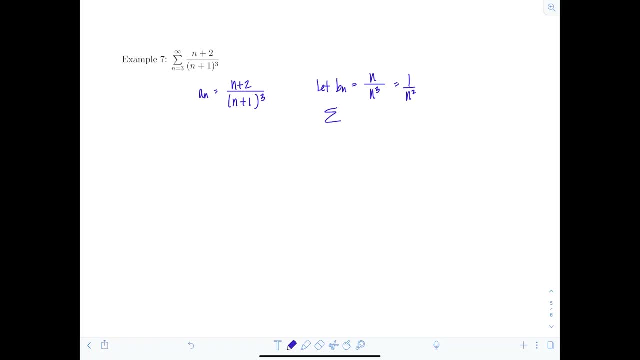 This is just a sequence. You have to write out a series: The sum n equals 3 to infinity of bn, which is the sum n equals 3 to infinity of 1 over n squared. Now I can say: oh, this is a p-series. 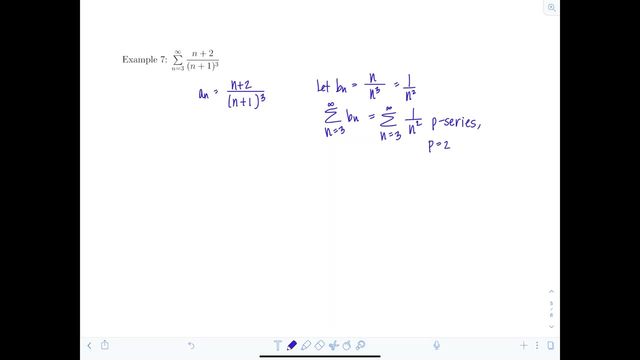 I have to also identify p. p is 2,, which is greater than 1,, which means it's convergent. Okay, Alright, so I don't have to show any sort of inequalities. I'm just going to take the limit, as n goes to infinity. 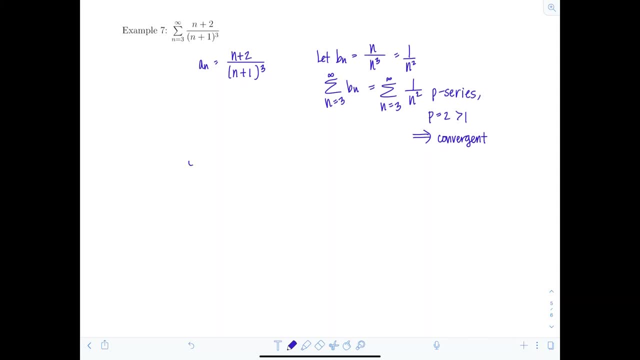 of the ratio of these terms and hope I get a constant. So limit as n approaches infinity of an over bn is going to be the limit as n approaches infinity an. an is n plus 2 over n plus 1, cubed over where's bn. 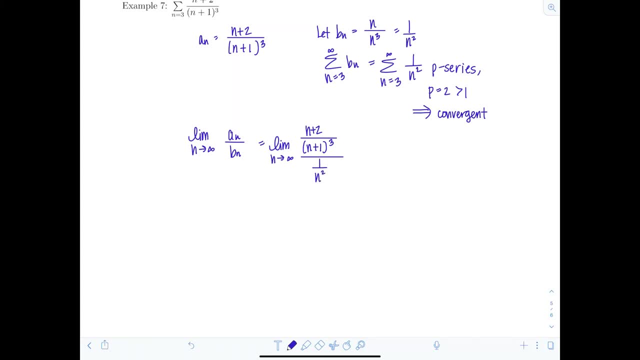 1 over n squared. Okay. So, cleaning this up, the n squared is going to come up to the numerator, So I have limit n approaches infinity n squared times: n plus 2 over n plus 1 cubed. Okay, If you need to distribute. 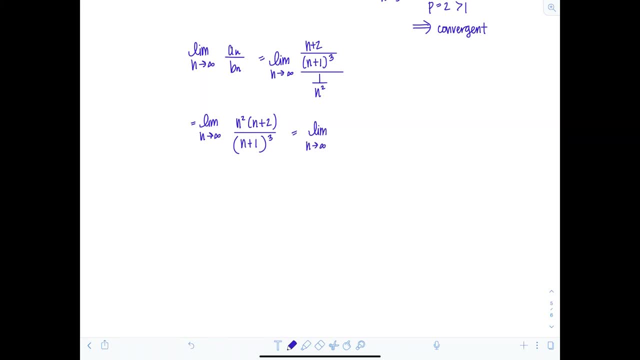 go for it. So this is the limit. n approaches infinity, Just in the numerator. Don't multiply out that denominator, That would be horrific. So n cubed plus 2n squared over n plus 1 cubed. Okay, so to take this limit. 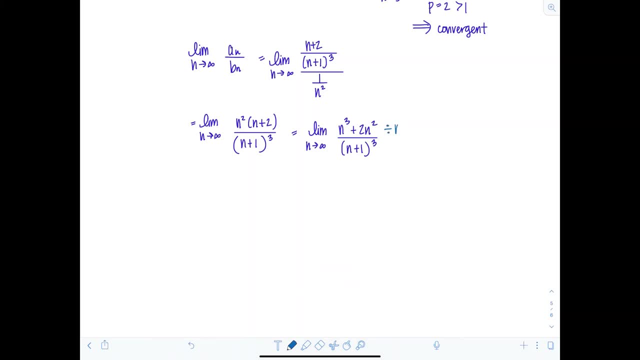 I'm going to divide out by the highest power of n in the denominator. So I'm going to divide by n cubed, divide by n cubed. So we have here: limit n approaches infinity. What's going on in the numerator? We got a 1 plus. 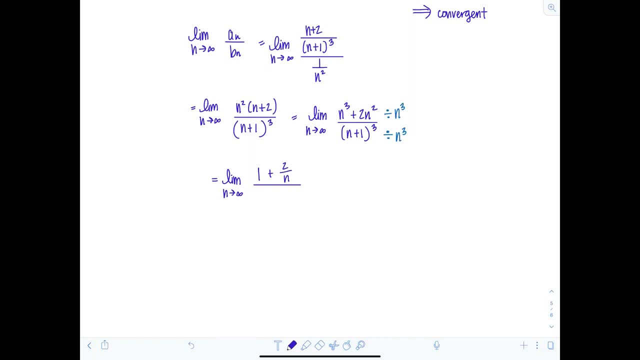 2 over n. Yes, Now if I bring that n cubed, I'm dividing by it inside the parentheses. I'm going to have 1 plus 1 over n, all cubed. Okay, if n goes to infinity in the numerator, 1 is 1, that's a constant. 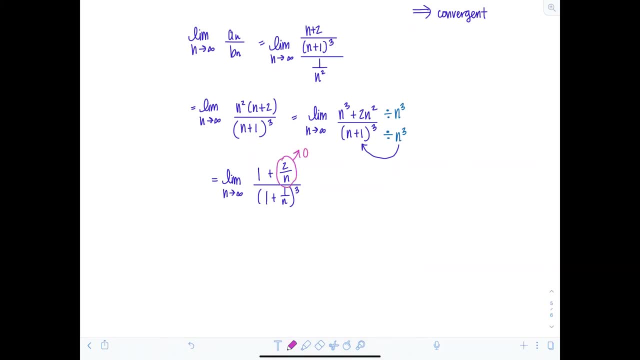 2 over n. that's going to go to 0.. And then I have 1 plus 1 over n. this is going to 0. So I'm left with 1 over 1, which is not negative, not 0,.